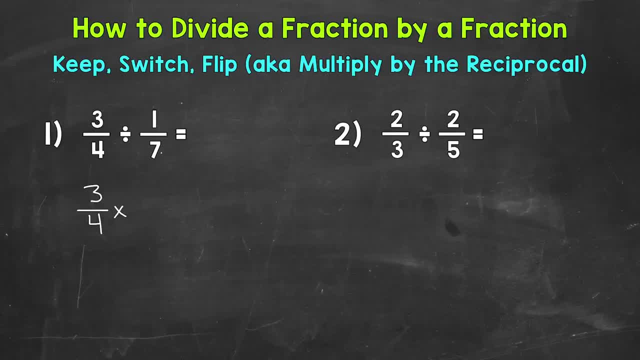 we're going to flip The second fraction, So the seven is going to be our numerator and the one is going to be our denominator. So we end up with seven over one. Once we get to this point, it's a multiplying fractions problem. 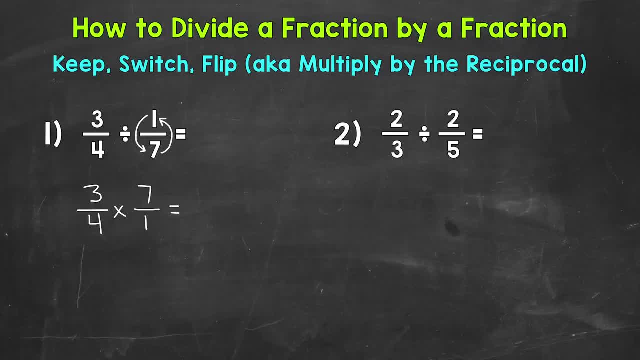 So we can multiply straight across: Three times seven is twenty-one, And then four times one is four, And we end up with twenty-one-fourths. Now, that's an improper fraction, so we do not want to leave it. We need to divide our numerator of twenty-one by four. 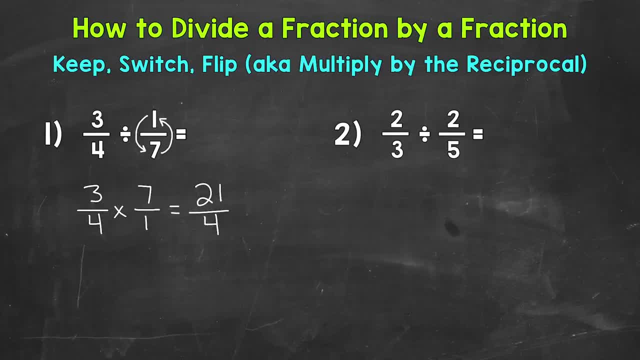 How many whole groups of four are in twenty-one? Well, five That gets us to twenty. So five whole groups of four, that's our whole number of the mixed number here. Now, that doesn't hit twenty-one exactly. We have a remainder of one. so that's our numerator in our fractional part of the mixed number. 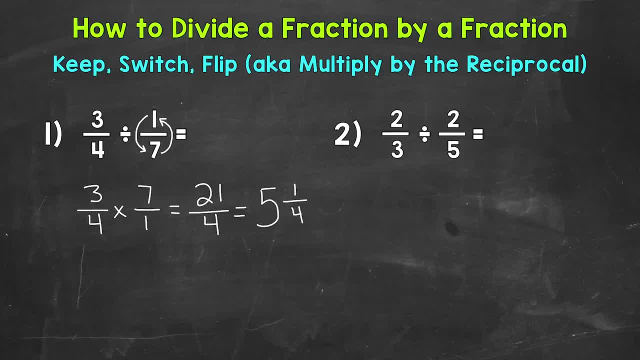 And we keep our denominator of four the same. Always look to see if you can simplify the fractional part of a mixed number. One-fourth is in simplest form. so we are done. Five and one-fourth is our answer for number one. 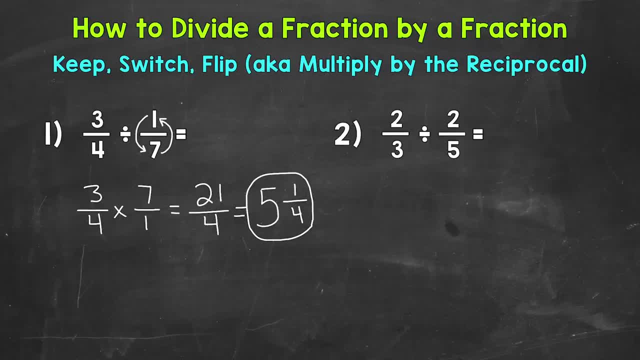 So three-fourths divided by one-seventh equals five and one-fourth. Let's move on to number two, where we have two-thirds divided by two-fourths. Keep, switch, flip. So keep two-thirds here, switch the multiplication and then flip that second fraction. 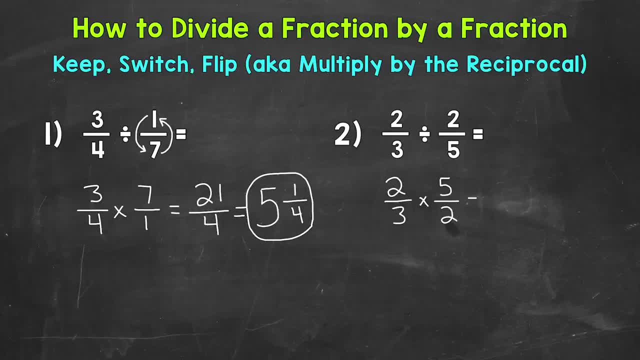 So five over two. And now we can multiply straight across: Two times five is ten, Three times two is six, So we get ten-sixths. So that's an improper fraction. For an improper fraction we need to convert to a mixed number. 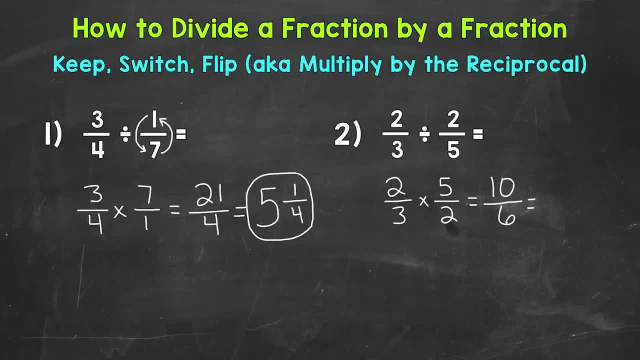 So ten divided by six, How many whole groups of six out of ten? Well, one, And we get a remainder of four. Keep our denominator of six the same. We can simplify four-sixths. We have a common factor of two. So let's divide each of these by two here. 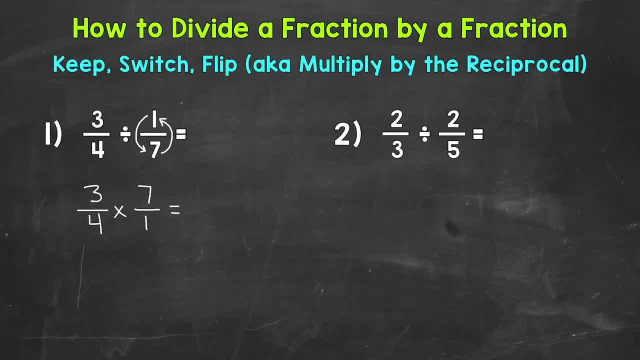 So we can multiply straight across: Three times seven is twenty-one, And then four times one is four, And we end up with twenty-one-fourths. Now, that's an improper fraction, so we do not want to leave it. We need to divide our numerator of twenty-one by four. 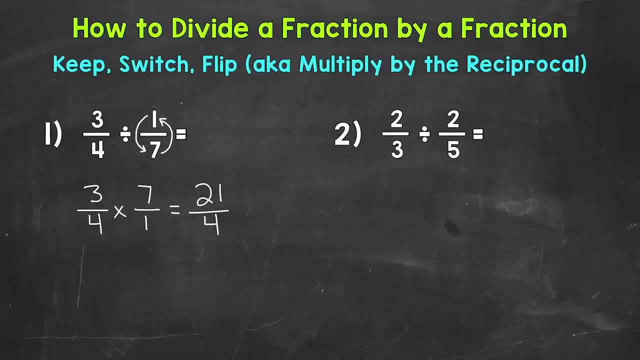 How many whole groups of four are in twenty-one? Well, five That gets us to twenty. So five whole groups of four, that's our whole number of the mixed number here. Now, that doesn't hit twenty-one exactly. We have a remainder of one. so that's our numerator in our fractional part of the mixed number. 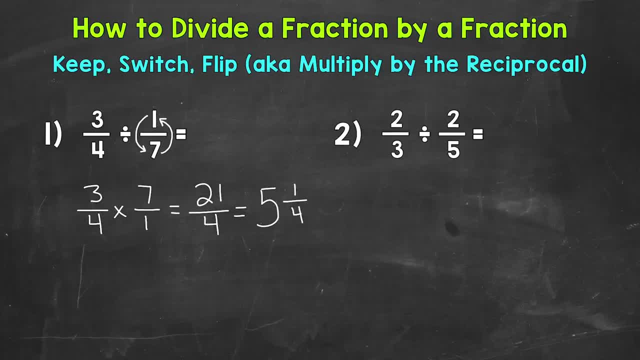 And we keep our denominator of four the same. Always look to see if you can simplify the fractional part of a mixed number. One-fourth is in simplest form. So we are done. Five and one-fourth is our answer for number one. 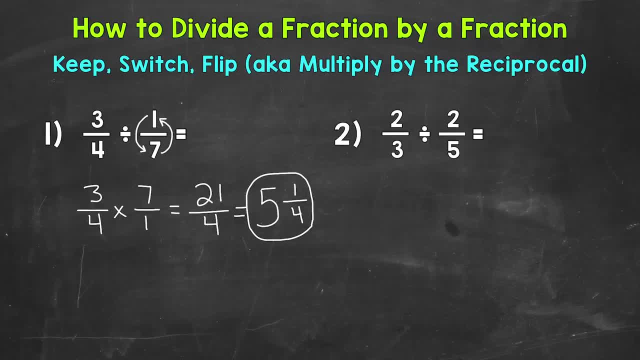 So three-fourths divided by one-seventh equals five and one-fourth. Let's move on to number two, where we have two-thirds divided by two-fourths. Let's move on to number two, where we have two-thirds divided by two-fourths. 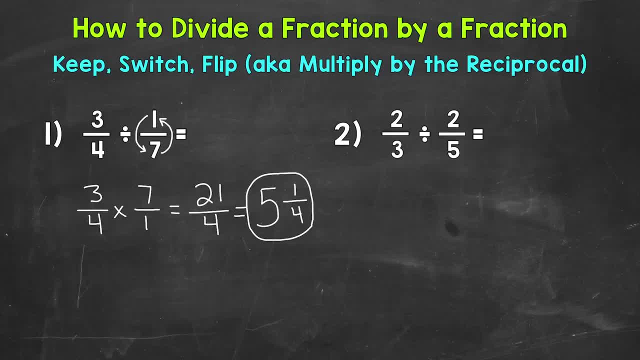 Keep, switch, flip. So keep two-thirds here, Switch the multiplication and then flip that second fraction, So five over two. And now we can multiply straight across. Two times five is ten, Three times two is six, So we get ten-sixths. 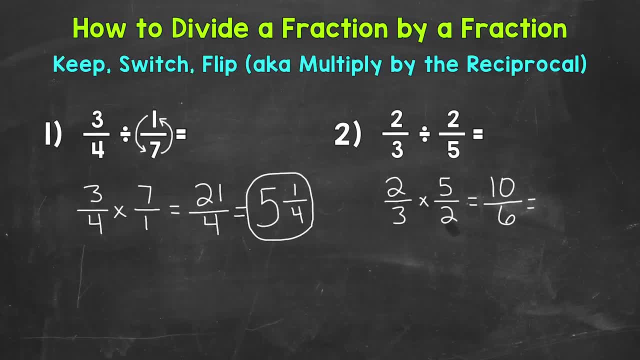 So that's an improper fraction We need to convert to a mixed number. So ten divided by six, How many whole groups of six out of ten? Well, one, And we get a remainder of four. Keep our denominator of six the same. 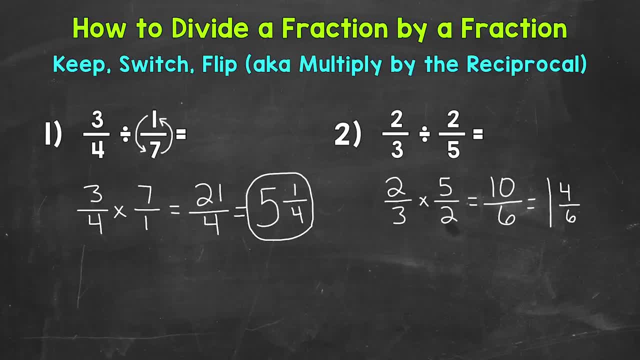 We can simplify four-sixths. We have a common factor of two, So let's divide each of these by two here And we get one and two-thirds. So our answer for number two is one and two-thirds. Two-thirds divided by two-fifths equals one and two-thirds.